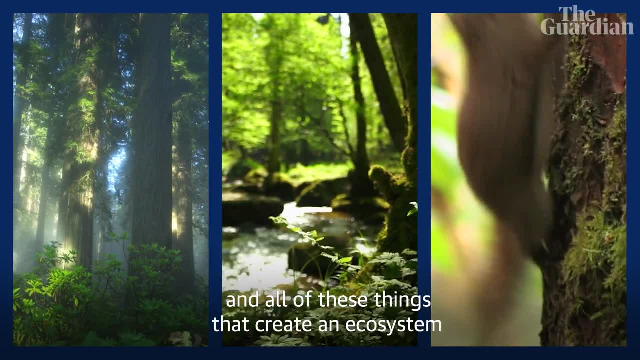 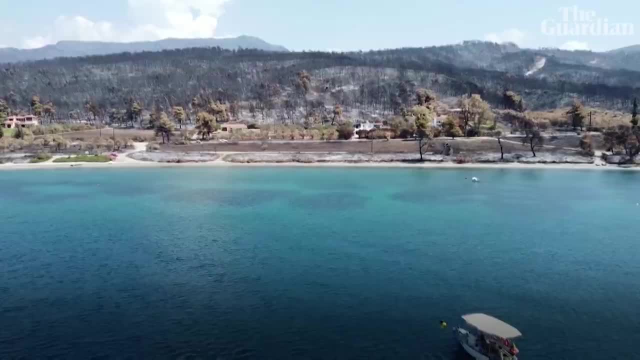 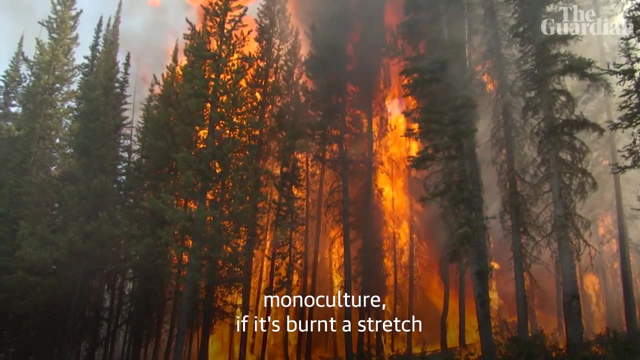 Mosses and animals and streams and all of these things that create an ecosystem are actually very strong and resilient when they're together. When you strip that all away, if you just take out all of the biodiversity, you're making the forest more vulnerable Once the fire's got hold of a 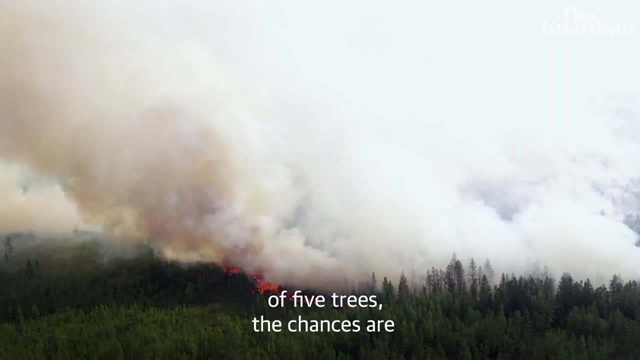 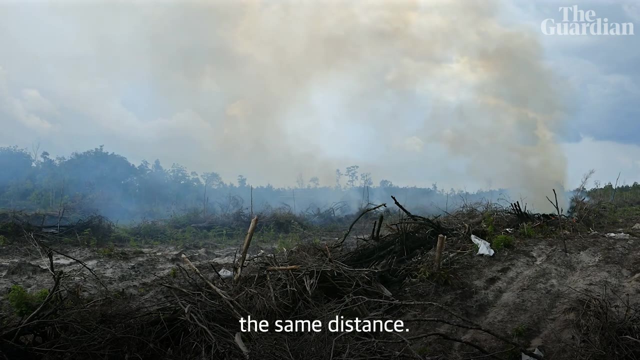 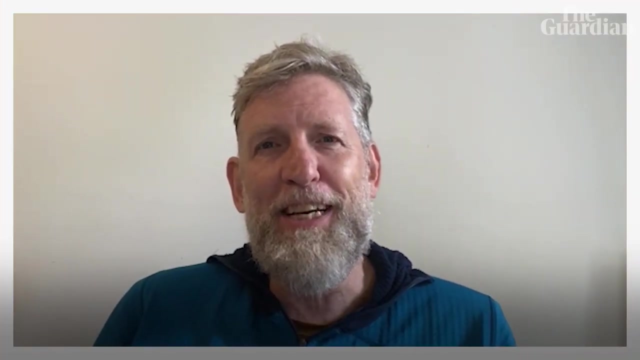 monoculture. if it's burnt a stretch of five trees, the chances are it can burn 5,000 trees because they're all planted in lines at roughly the same distance. Counter-intuitively, there are actually fewer wildfires than there were in the past. 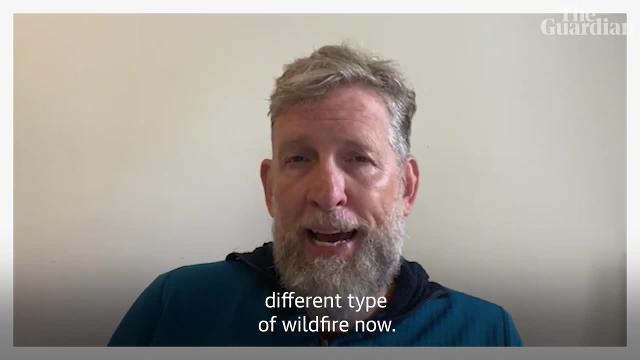 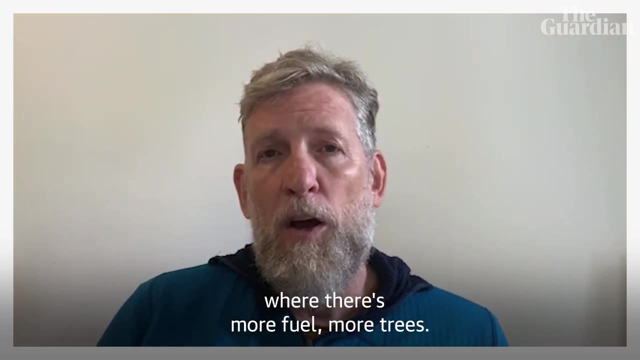 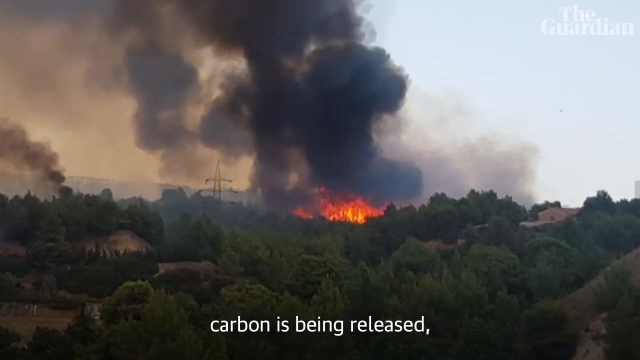 But what's happening is that there's a different type of wildfire now. We're seeing fewer fires but more intense ones, because fires are spreading to areas where there's more fuel, more trees, And when trees burn, obviously much more carbon is being released and they burn much longer. 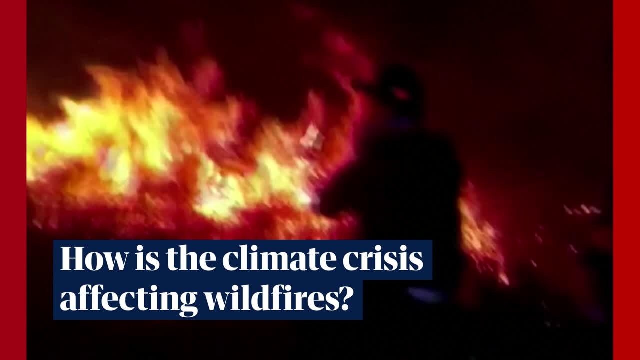 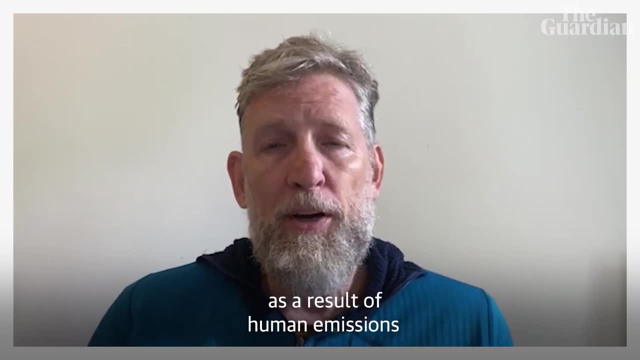 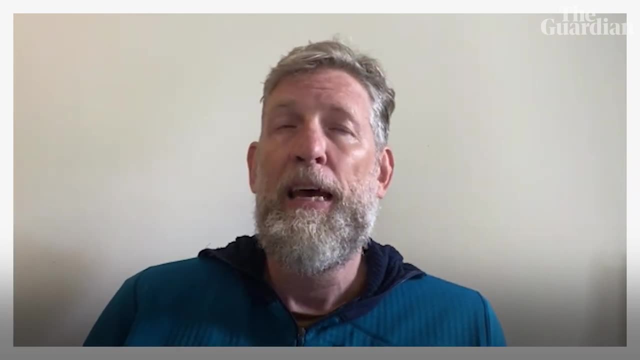 and much harder. We've already had more than one degree Celsius warming since the industrial era as a result of human emissions like exhaust fumes, industrial releases from chimneys and deforestation, And all of these gases are being released into the atmosphere. That's kind of cloaking the planet. 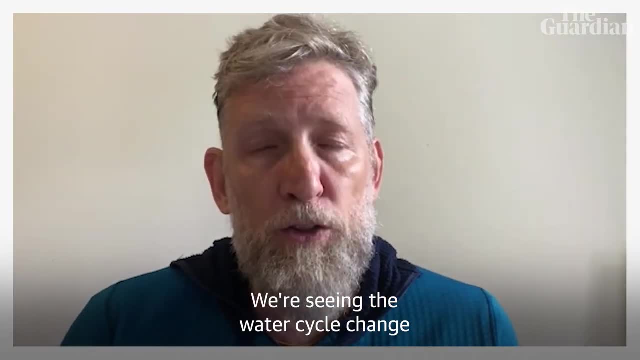 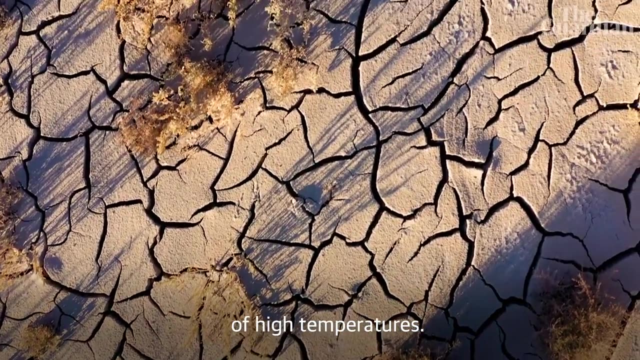 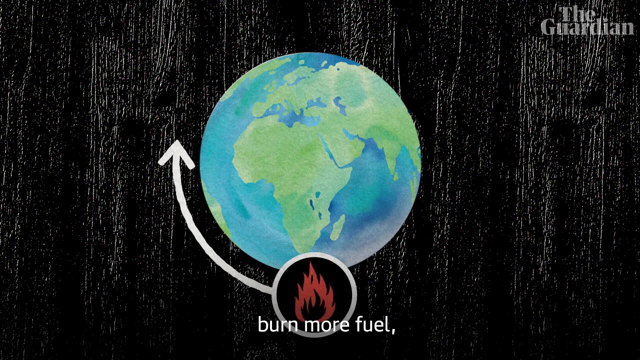 And then everything below it heats up. We're seeing the water cycle change and we're seeing the lands dry out more frequently, And protracted periods of high temperatures are kind of a reinforcing climate feedback mechanism, because as more fires burn, more fuel, they release more carbon into the atmosphere. 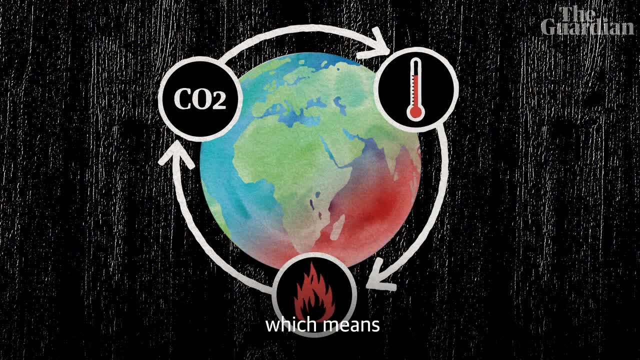 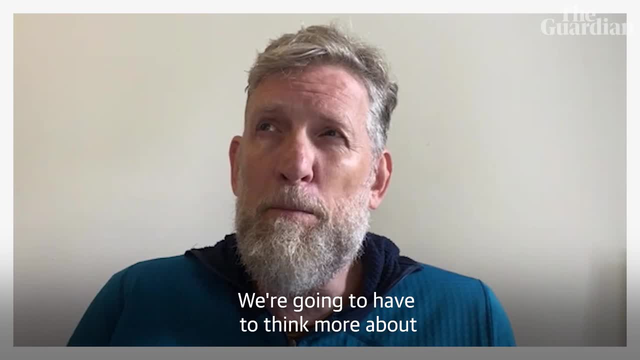 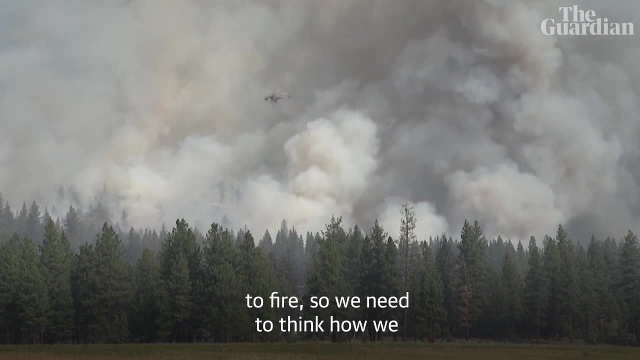 which means more global heating, which means more fires. We're going to have to think more about natural defenses, because plantations and monocultures are much more vulnerable to climate change. So one of the things we need to think about is the future of nature and the future of the environment. 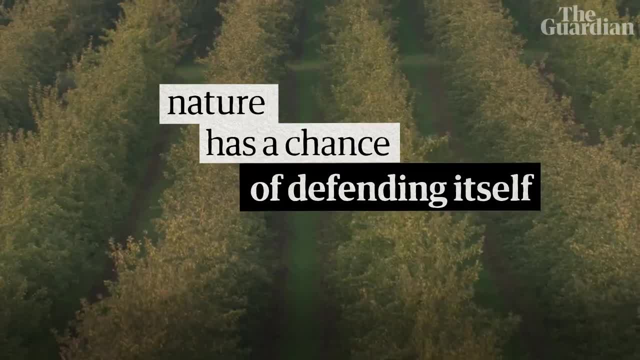 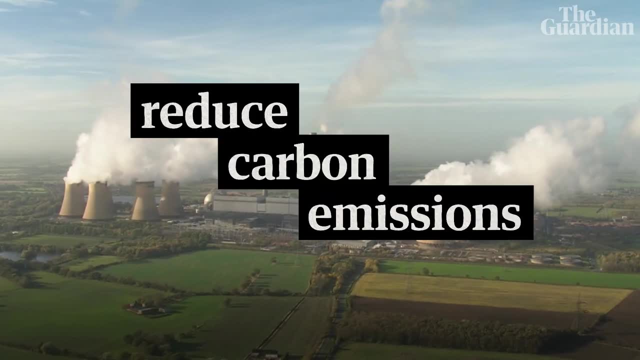 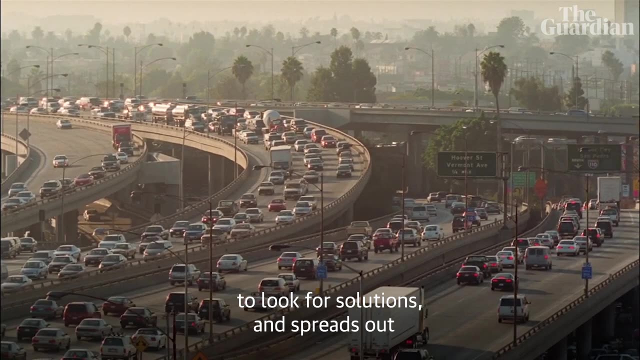 We need to think about how we plant things so that nature has a chance of defending itself. At the same time, the best and biggest thing we can do is reduce carbon emissions as quickly as possible. At the very least, that buys more time to look for solutions and spreads out the impact.